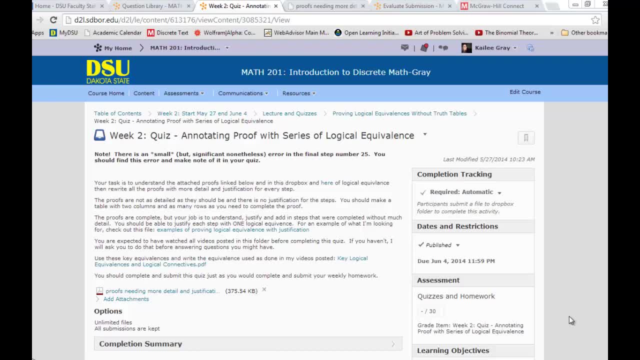 just submit it. so I just want to see if you learn something and you're able to understand what's happening with each of these steps. so a file that you definitely want to have open while you're completing. this is the key certification. a form of course study is probably referring to taking a. 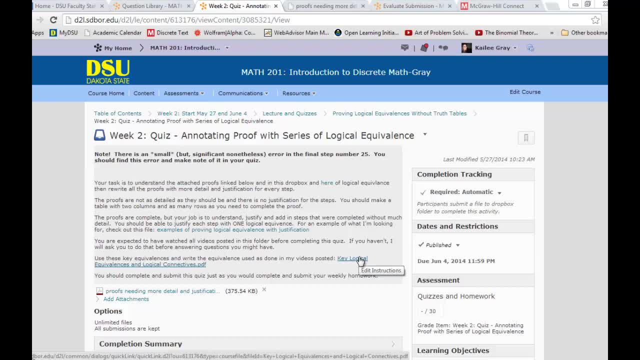 draft data test and from that one you go back into big letter, you're gonna move up the type and load in and up dot dot all because every класс is gonna tab with their own things, different ways ofnaj, and so you want to talk about best practices and what's changing with yourprised testING and your law. 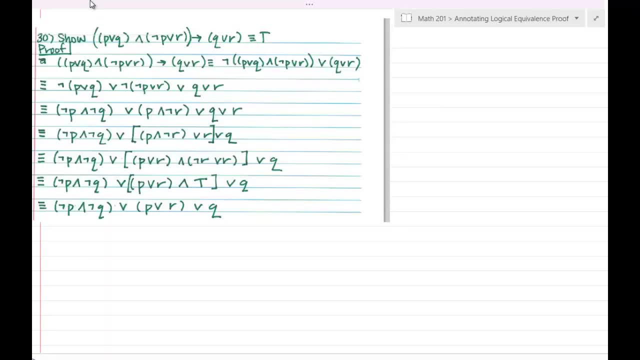 problem. so once you're ready, it's actually really the time stage to start interacting, if you're warm about getting those log to do questions on your text as a bouquet or to favorite items to care about. to talk through just a few of these steps here to help you understand what. 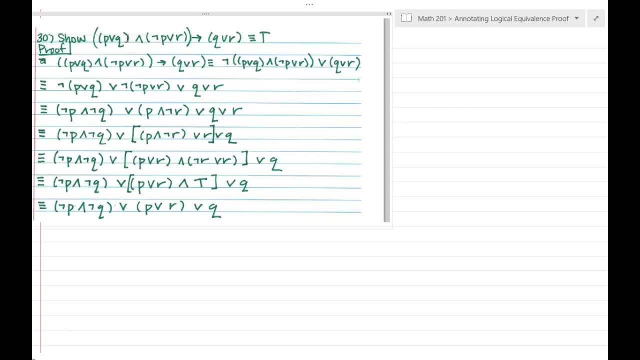 I'm looking for. so number 30. we're trying to show, we're trying to prove that some compound proposition is a tautology. so it looks like we're. you know, starting on the left hand side and applying the equivalence that P implies Q is logically equivalent to not P or Q. so hypothesis implies, conclusion is: 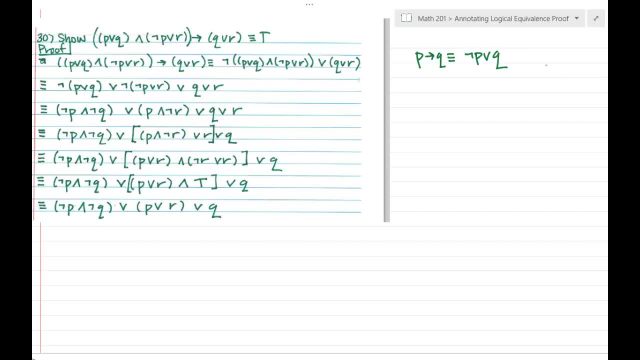 logically equivalent to the negation of the hypothesis or conclusion. so keep that in mind. but let's just- yeah, let's just go step by step see if we can follow along here. and that I mean, you're basically just going to be rewriting what's already done, but the only difference is you're going to also be 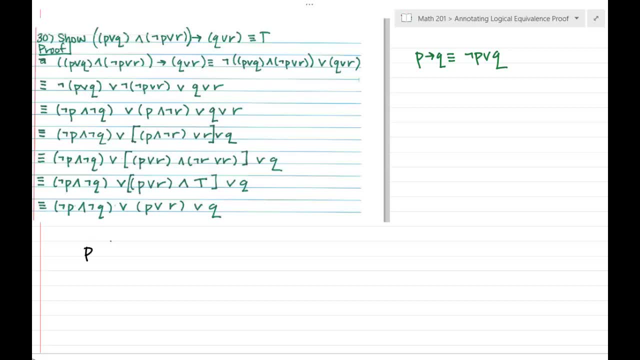 writing the justification for each step, and all I'm looking for with the justification is the justification for the evaluation. so this is going to do it. justification is just some logical equivalence that you're applying. that's in the list of those key logical equivalences, and so obviously there's. 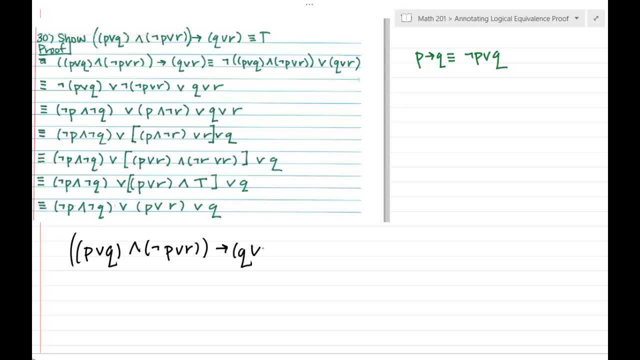 different ways to approach this problem, but since the works already done with for you, go ahead and just follow along with with the given steps that you have. so this first step that I'm writing down, this is just our beginning point. I'm just copying down the left-hand side, beginning the next one there. so this is. 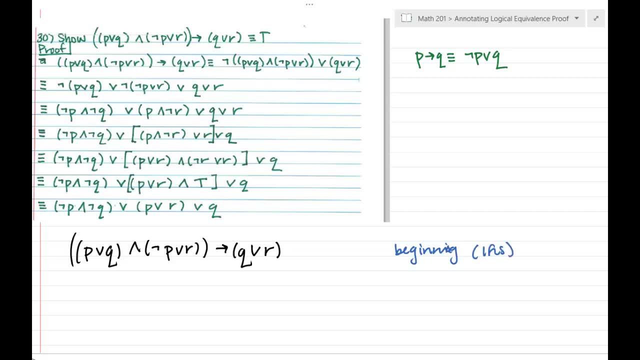 the left-hand side of my problem. okay, so I'm just copying down now the next step and- and while you're doing this you kind of have to reason through this: is the next step reasonable, or is there too many things happening at once? I think for the most part, each of the steps is broken down pretty well for you already. 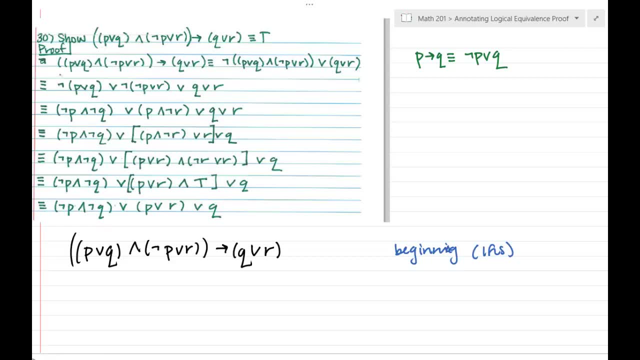 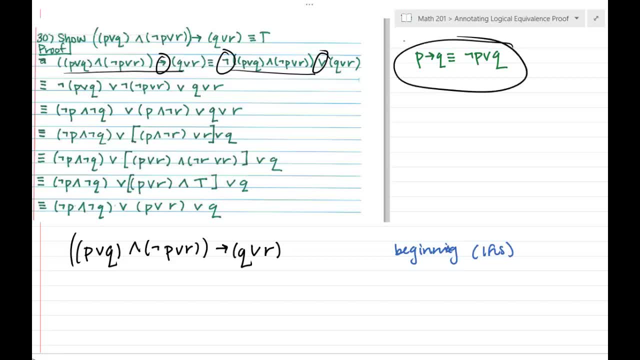 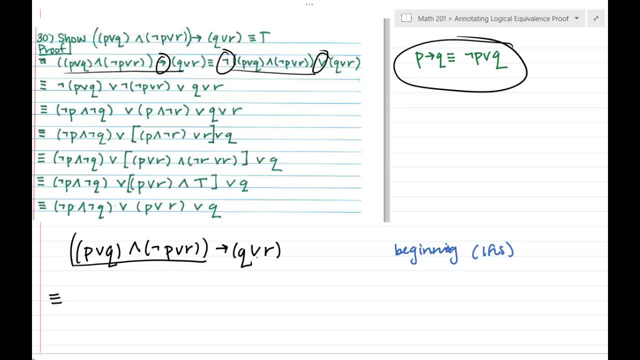 did is I look at this and I said: this is my hypothesis, this is my conclusion. so I negate the hypothesis and then or conclusion: okay, so I'd write down that first step and then all I do is just write down my justification here. so I'm going to write down. write down my justification here. is that P? 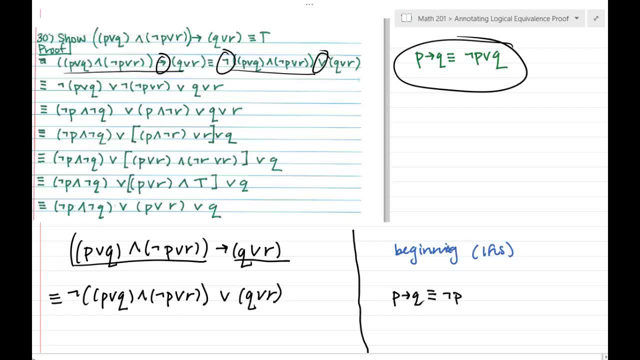 implies Q is logically equivalent to not P or Q. all right, so let's see what happens next. okay, now what's happening is: this: negation is being distributed, so we've got De Morgan's laws happening here. so I'm going to go ahead and do that step. but instead of just writing down that step, I'm going to add in the 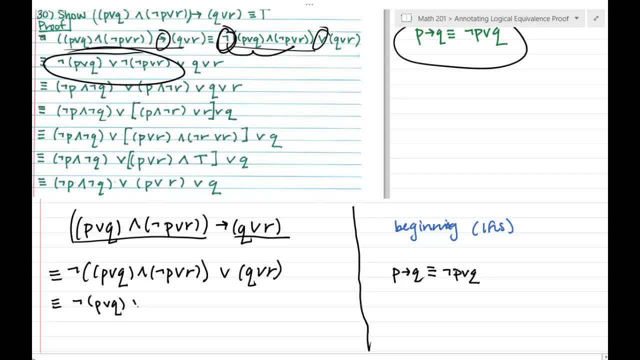 justification. so I know that what I did was just take two propositions joined by and, and negate both of them, change that middle one to an, or so I used De Morgan's laws, and that's just that. the negation of P and Q is logically equivalent to the. 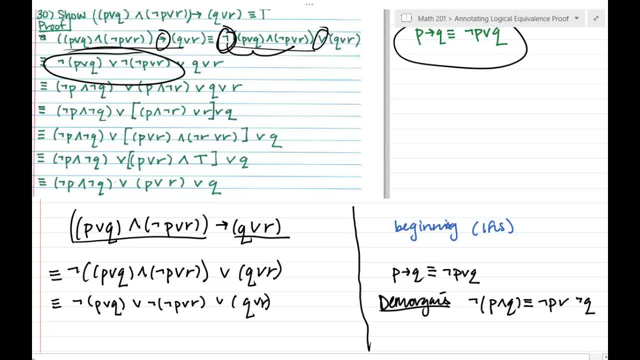 negation of P or negation of Q. so now let's see what happens. okay, now, this is an example where there's quite a few things happening here more than I would like to see what's happening. it looks like there's De Morgan's laws happening on this piece and on this. 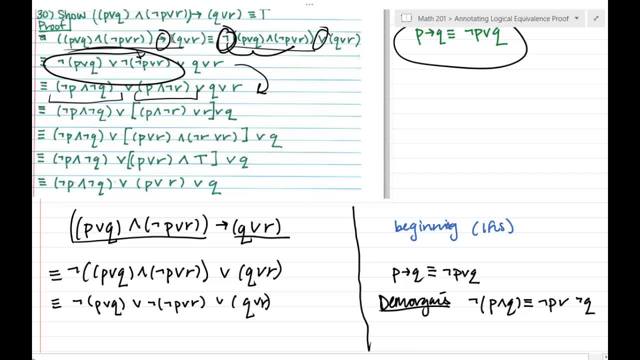 piece and double negation. okay, so only only one justification per step. okay, don't get crazy on your steps. I promise you it's. it's for the better in the end. okay, so what I'm going to do is split that into a couple steps, so I'm gonna apply. 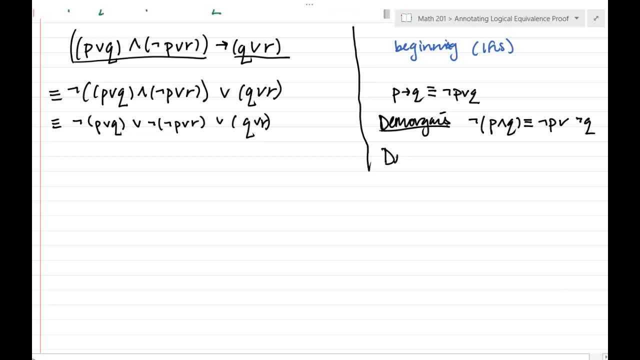 De Morgan's over and or so we've got De Morgan's law. if I negate two propositions joined by, or, I'm going to negate both pieces and change it to an and, so that I'll apply on this first and second piece, so not P and not Q, or now. 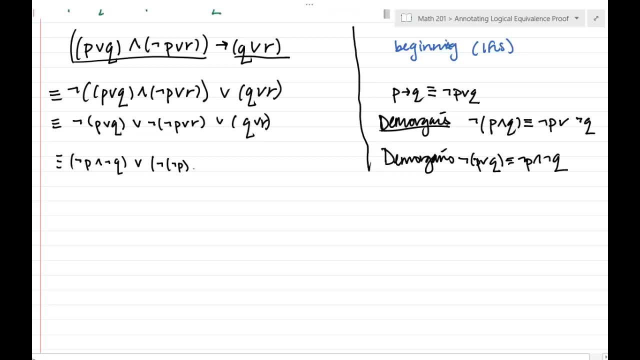 I'm gonna write not, not P, because I'm gonna need another justification here for any alteration to that. okay, or Q or R. okay, so now I'm gonna use double negation, double negation, and you don't have to write De Morgan's double negation, all I'm looking. 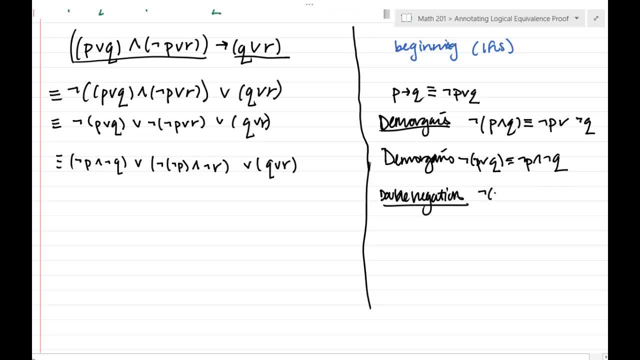 for on each step is the general form of that logical equivalence that you're using. so, whatever appears in that key logical equivalence document, that's what I want you to write down for the justification. okay, and make sure you're clear on what's justification and what steps, okay. 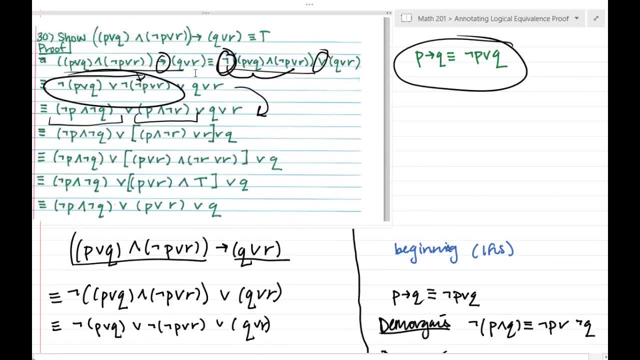 all right. so now let's see what happens next so we're able to get here. we got this there and then it looks like we've got a few rearranging going on right. it looks like Q and R changes places, change places, and then it looks like we have. 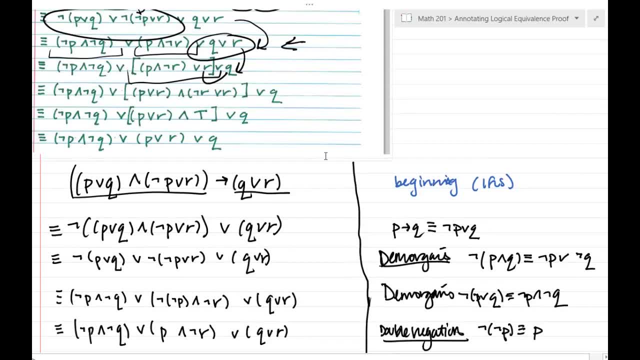 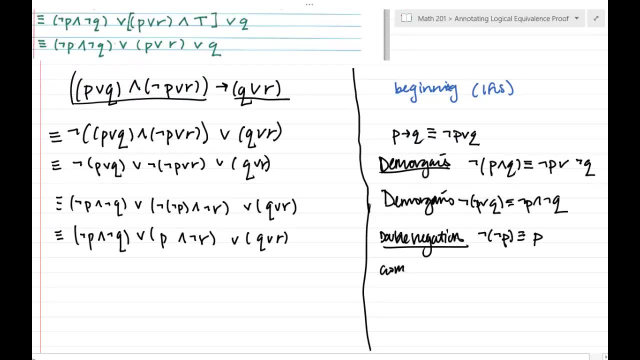 some associative stuff going on. so what I'm gonna do to get to that point eventually, I'm gonna break it down to a couple steps. so I'm gonna use the commutative law for or to switch the order of Q or R. so I know that the order that I do, the or, does not matter as long as I've got. 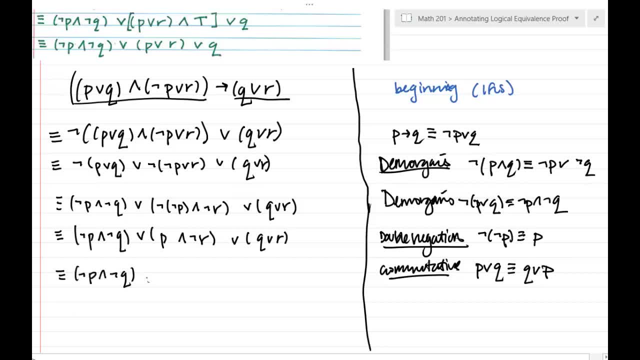 the same operator and I'm not moving more than one thing at a time and I'm definitely not trying to waste your time. so use your judgments and and do what you think is best here, but I do think it's a good practice just to write this. 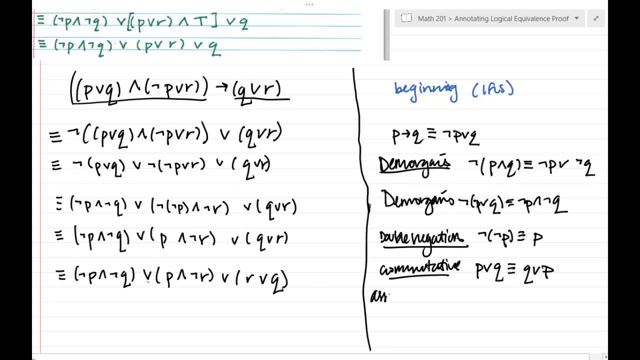 out and take your time. so associative laws, I'm gonna write: let's see if I've got P or Q or R. This is logically equivalent to P or Q or R, because somehow I want to group this R together. so I'm going to use associative laws to do that. So not P and not Q or P and. 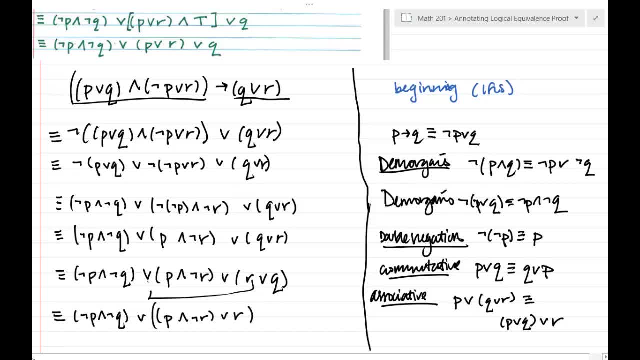 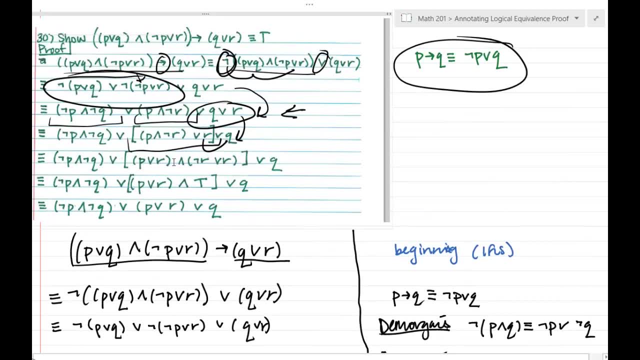 not R, because I want to put that R with the negation of R. so that's why I'm trying to group those together. And then it looks like I've got some distribution happening. So after I group that R by the piece I want it with, it looks like I'm distributing over an AND. 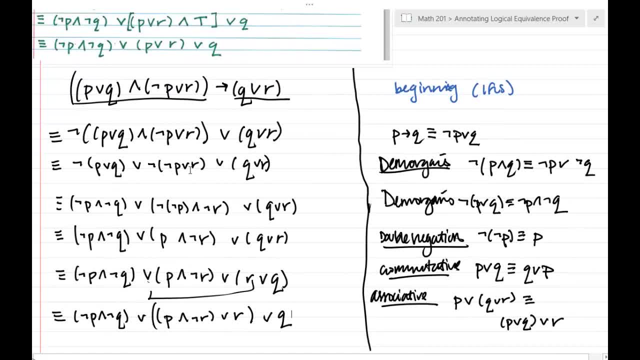 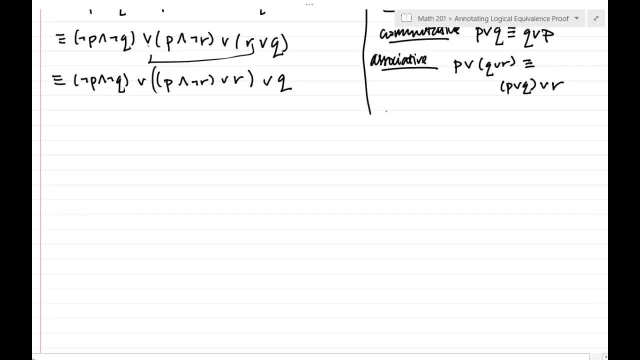 with an OR. so I would just write out that distributive property that I'm using here. So in this next step I'm using the fact that if I take P and Q OR R, This is the same. and this is all on that key logical equivalence sheet. So that's where you're going to find all this stuff. 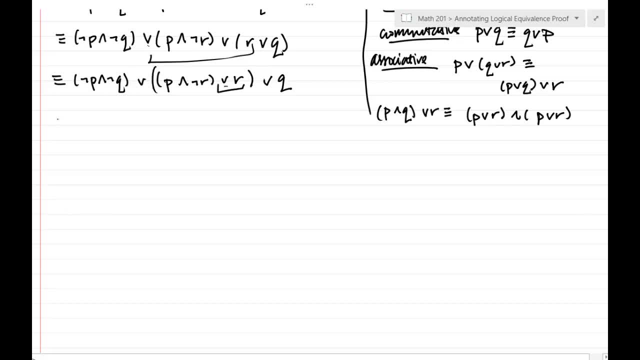 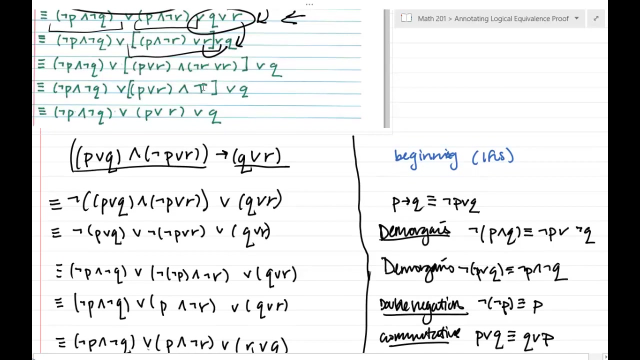 So I'm taking OR R and distributing it to both pieces, P OR R and NOT R OR R- Now I have some work to do with that. NOT R. I know that that's logically equivalent to TRUE, so that's how we got there. 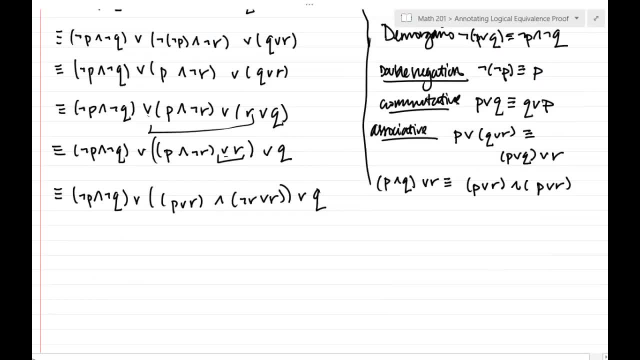 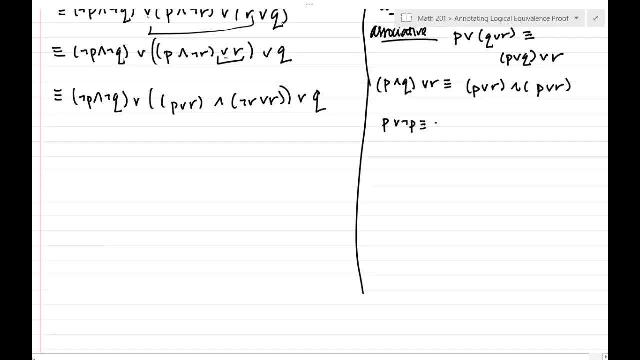 If I take- and that's another equivalence, that's on that sheet- if I take P or NOT P, or if I take NOT P or P, I'm going to get a TRUE statement. And that's just because P and NOT P are always going to have opposite truth values. 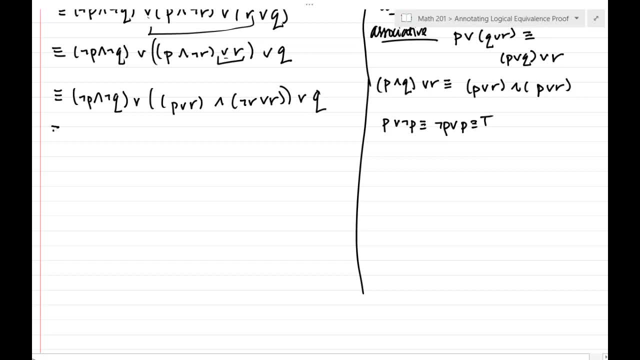 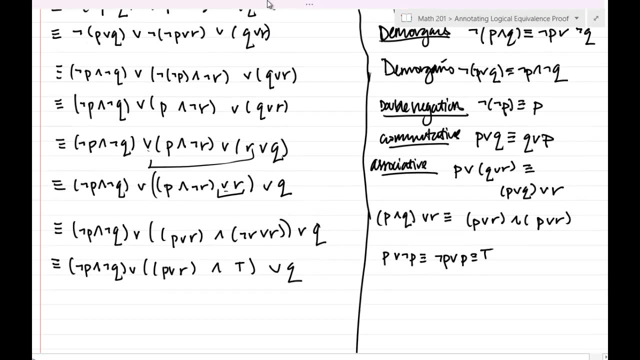 With the OR operator. you only need one to be TRUE to have an overall TRUE statement. So I'm going to have P OR R AND TRUE OR Q. Okay, it looks like just one more step here that I'm going to show you, and it's not quite done, but hopefully it gives you a little bit of direction.